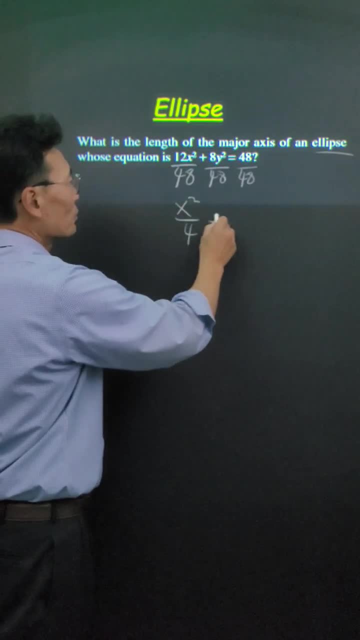 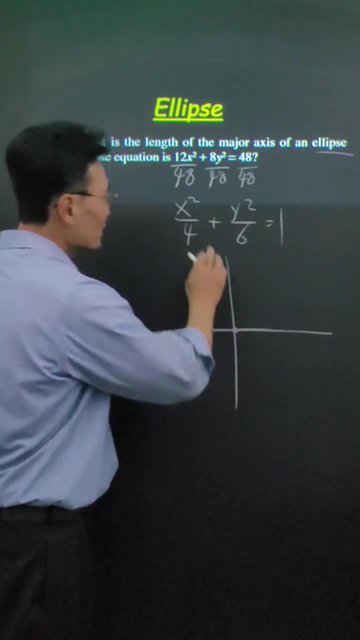 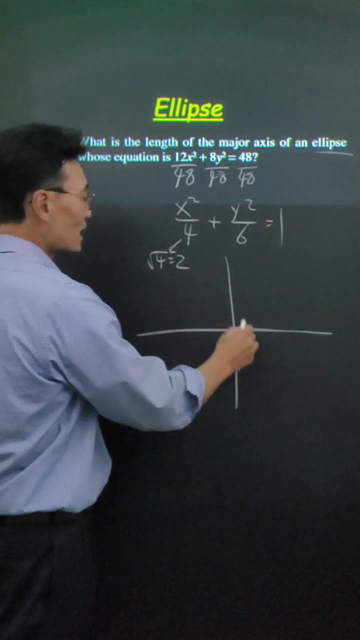 It simplifies to: x squared over 4 plus y squared over 6 equals to 1.. Then the center will be at 0, 0, because we only have x squared and y squared on the top. Then, if you take the number underneath the x squared, take the square root of that and that's how far we're going to go to the right and how far we're going to go to the left. 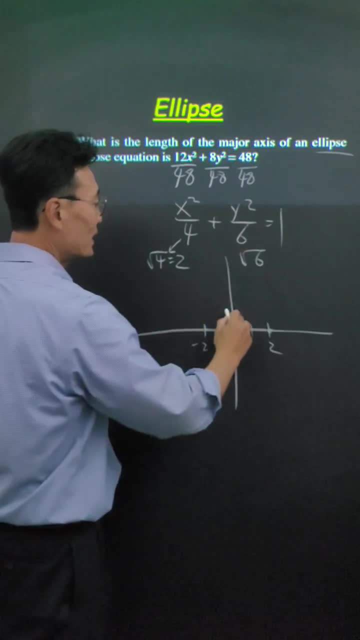 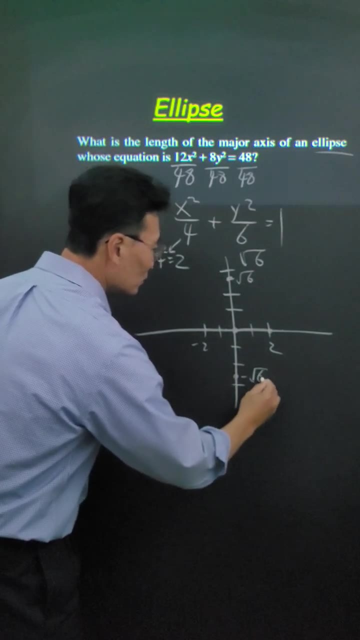 Then take the number underneath the y squared, take the square root of that and that's how far we're going to go up and that's how far we're going to go down. for the vertices, If we connect the dots, then we get our ellipse. 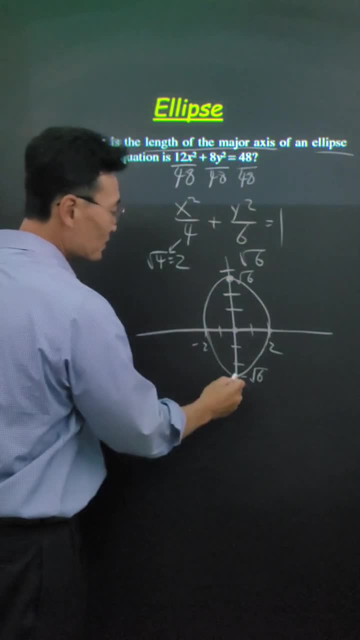 The length of the major axis will be the distance from the vertices on the top and the bottom. That's the longer way and it's going to be 2 root 6.. 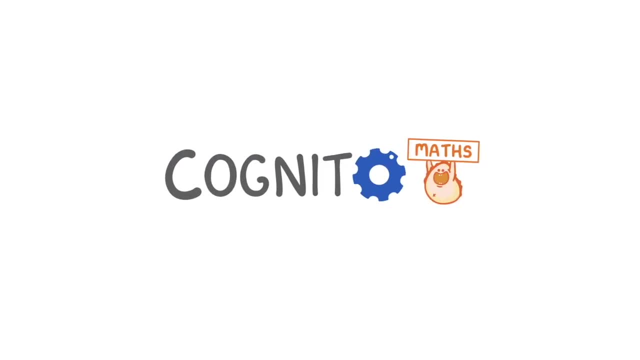 In this video, we're going to cover the basics of how we can simplify algebraic expressions where numbers and letters are being multiplied together, like in these examples. Now, the most important thing you need to know when you're doing algebra is that we generally don't write to the multiplication signs and instead 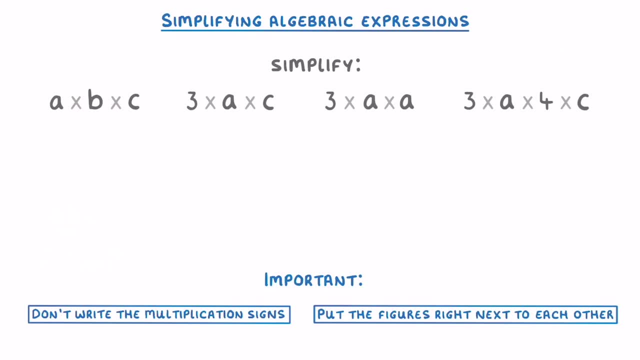 we just put the figures that are being multiplied together right next to each other. So for this first question, instead of writing a times b times c, we'd get rid of the multiplication signs so that we just have the a, the b and the c, and then we'd also get rid of the spaces in.